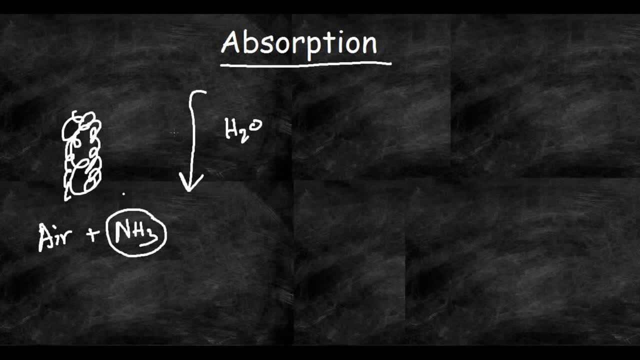 mixture to get the ammonia back. So that is what stripping is. So now we will discuss only absorption, where we will consider that I have a mixture of air and ammonia and I have to use water in order to absorb this ammonia from this air and ammonia system. So this is what we will. 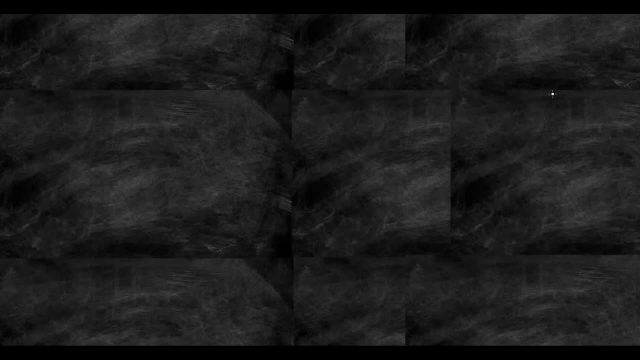 deal with. So here comes my absorber. So here comes my absorption tower. So from the bottom, from the bottom, the gas mixture will be pumped in. From the bottom the gas mixture will be pumped in. Now, the gas flow rate. the gas flow rate I will denote with G, Np, plus. 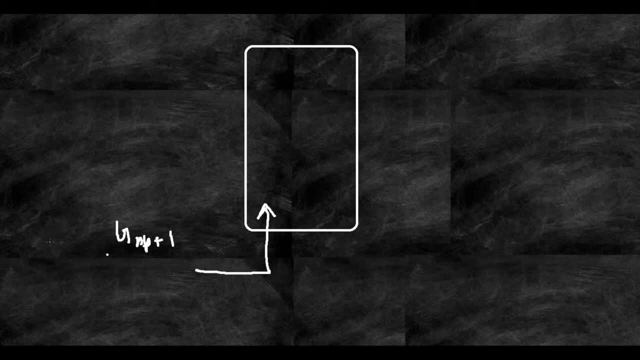 1. This is the gas flow rate. So this, the unit of this, will be kg- kgs per second, or kgs per hour, or the unit can also be kilo moles, kilo moles per second. So this is. 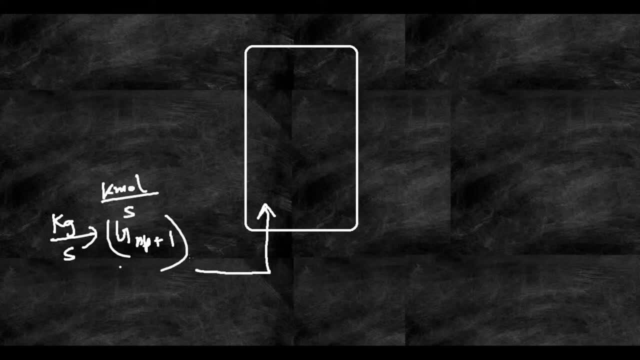 the unit of G Np plus 1.. So now the concentration or the mole fraction of ammonia in this ammonia air mixture. I will denote this with Y Np plus 1, Y Np plus 1.. This Y Np plus 1, this will be: 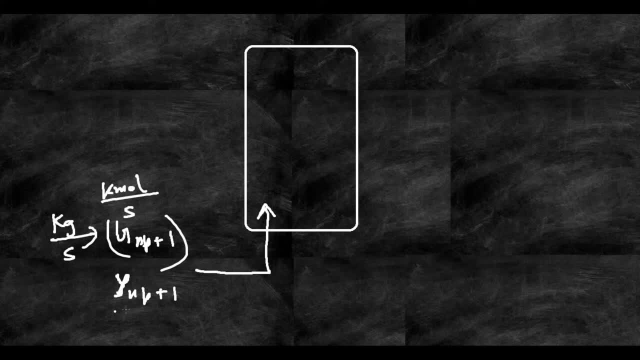 small letter y. This small letter Y, Np plus 1, is the mole fraction of ammonia in this ammonia air mixture. So this is pumped in from the bottom Now. this will move out of the tower. This will move out of the tower. 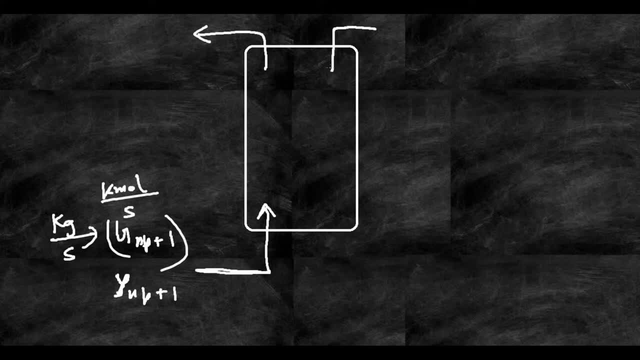 from the top, and also from the top i will put the desirable solvent. the desirable solvent will be water, over here now, the flow rate of the water, that is the kilo moles, kilo moles per second of water that i am putting in. i will denote this with l l naught. i will denote this with l naught. 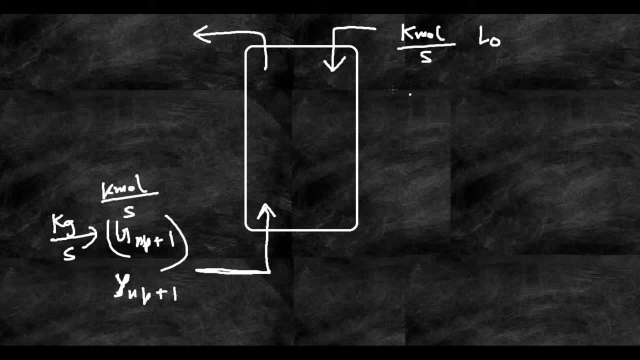 now, in most cases, the solvent which is put in does not contain any, any solute, that is, in this case, it will be a pure solvent, a pure solvent. so for a pure solvent, for a pure solvent, the concentration or the mole fraction of ammonia in this solvent will be nothing but zero. hence i will 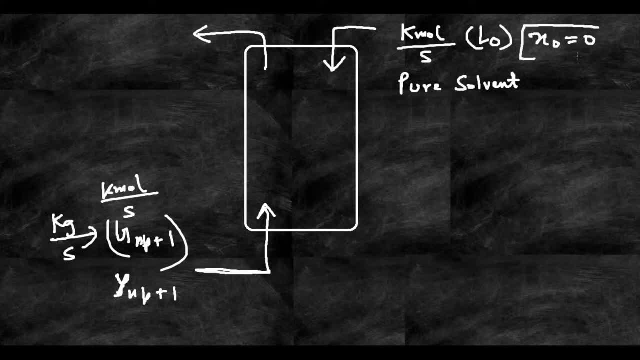 write: small x naught is equal to zero. small x naught is the mole fraction of ammonia in the solvent which i am supplying from the top. so this is equal to zero because i am considering pure solvent. if the solvent is not pure, then there will be some value of this x naught. so now what i do is: 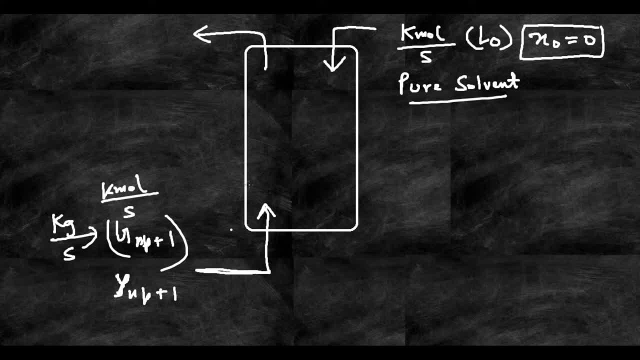 this water, you, this water, will go through the absorber. it will, it will come in contact, if it will come in contact with the air ammonia mixture which i am pumping from below, and it will absorb the ammonia from that mixture. so now, after absorbing, it will come down from this point. now, here i will again name: 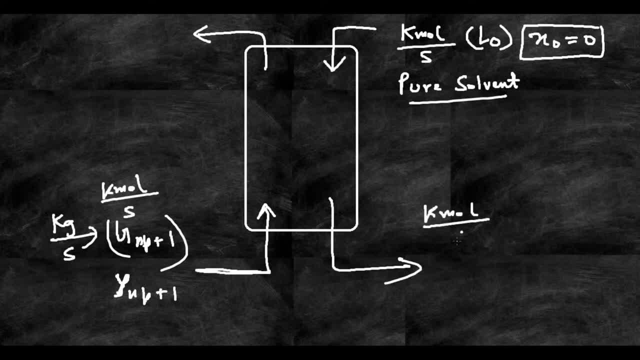 the flow rate, that is, kilo moles, kilo moles per second, of the mixture, which is of the solvent which is coming out. this i will name as l np. this is my l np and the concentration or the mole fraction, the mole fraction of ammonia in this stream will be higher because it has absorbed. 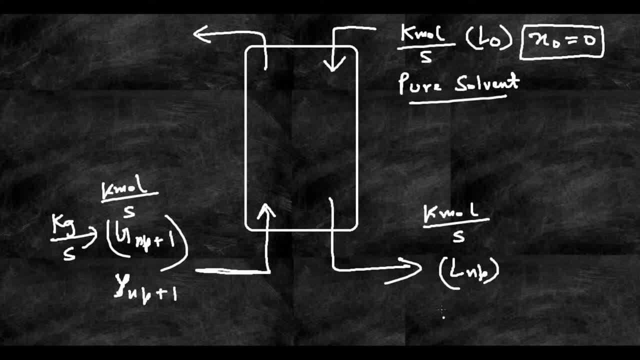 most of the ammonia which was flowing upwards. so now here i will name this as xnp- xnp. so what is xnp? xnp is the mole fraction of ammonia in this solvent at the bottom, that is, after the absorption has taken place. so now we will discuss a little bit about this top stream. 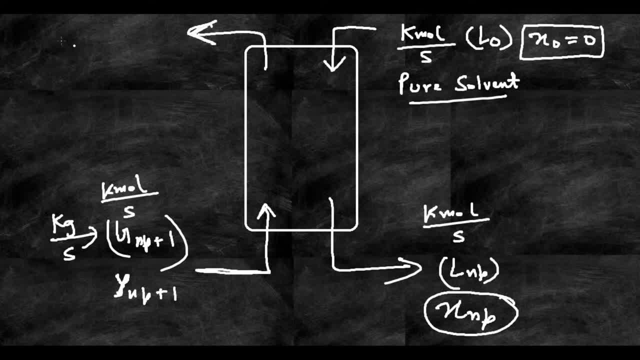 of this gas which is flowing out now in this gas stream. what will happen is the flow rate, that is, the mass flow rate, will be denoted by g1. this will be denoted by g1, so g1 is the kilo moles, kilo. 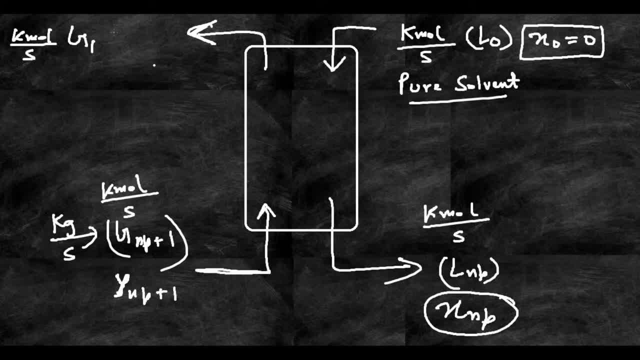 moles per second or kgs per second of the gas which is flowing out. that is the air ammonia mixture and also the concentration of ammonia, that is the mole. so the mole fraction of ammonia which is present in this exit gas stream after the absorption has taken place. i will denote this mole fraction with: 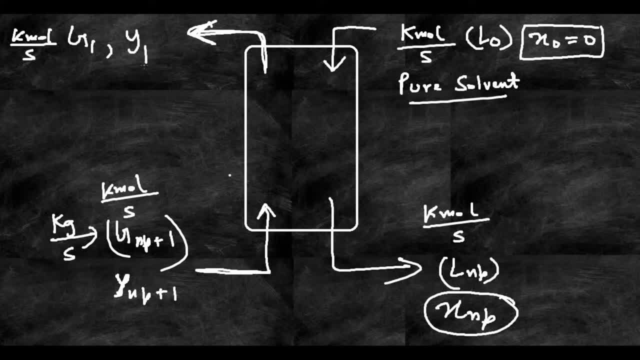 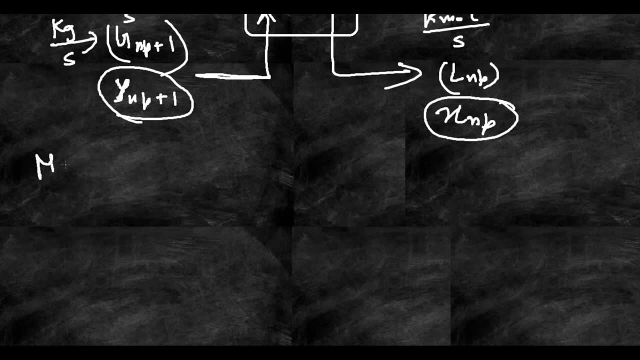 small y1. so now, one important thing which we need to know is all these things i have written are small letters, which means these are all mole fractions, but in equations we will need a quantity which is known as the mole ratio. so what is this mole ratio and mole fraction? it is very easy: mole ratios. 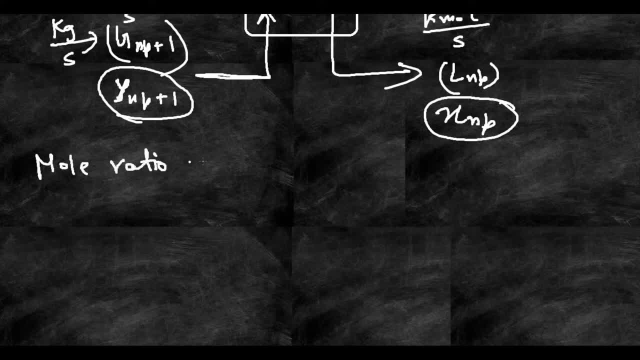 mole ratio. mole ratio i will denote with capital letter. so for mole ratio, if i am writing capital y, it means it means the moles of moles of ammonia present. moles of ammonia present. moles of ammonia present divided by rest of the moles. rest of moles. 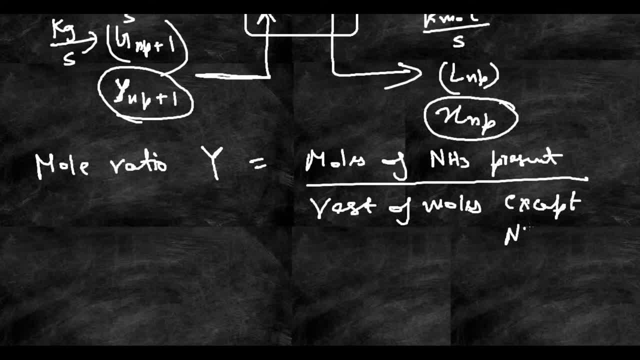 except except ammonia. so this is what mole ratio means, and when i am writing mole fraction may, when i am writing mole fraction, what i mean is- i will denote this with small y- so this will be equal to moles of moles of ammonia. moles of ammonia present divided by total moles. total moles. 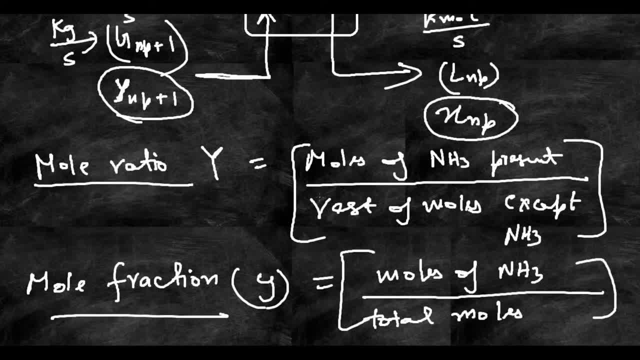 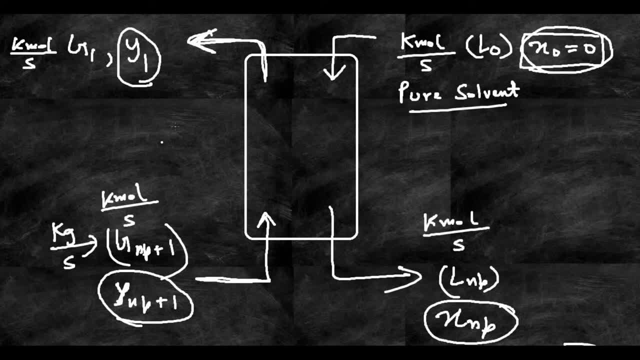 so this is the difference between mole ratio and mole fractions. we will live a little more in this, have a little more more of this mole ratio and if we move those moles, i should be able to understand this better as we proceed. so first we will deal with the 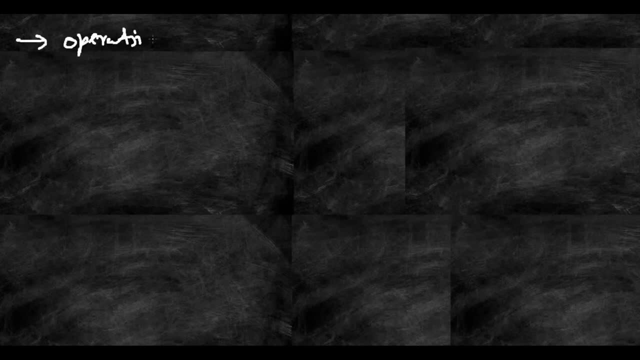 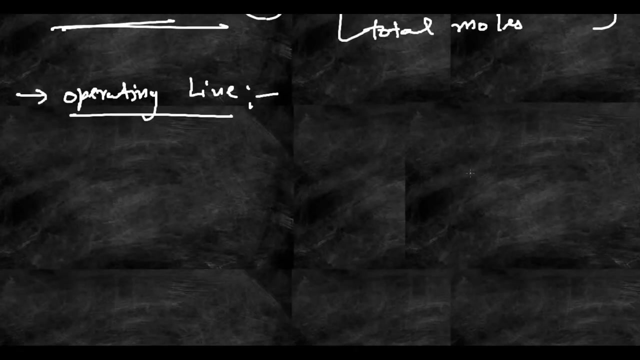 deal with obtaining the operating line equation. so to find the operating line equation, let me write absorber over here this is the absorber tower. so first we will try to derive the operating line equation, operating line, operating line equation and mole fractions. so i can write. i can write this relationship as, in order to convert from: 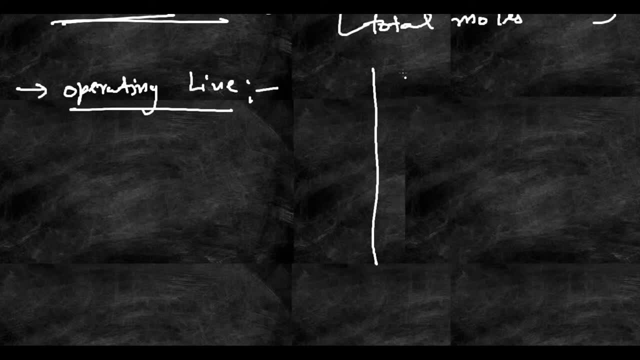 mole ratios to mole fractions. what i need to know is mole ratio. capital y is equal to mole fraction y divided by 1 minus y. this is how i can easily convert from mole ratio to mole fraction, where y is the mole fraction and capital y is the mole ratio. so remember this, because we will need this. 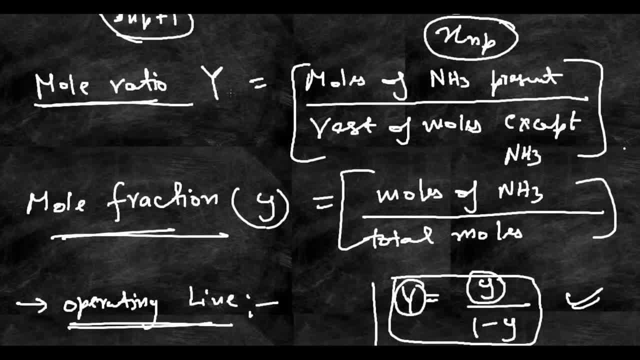 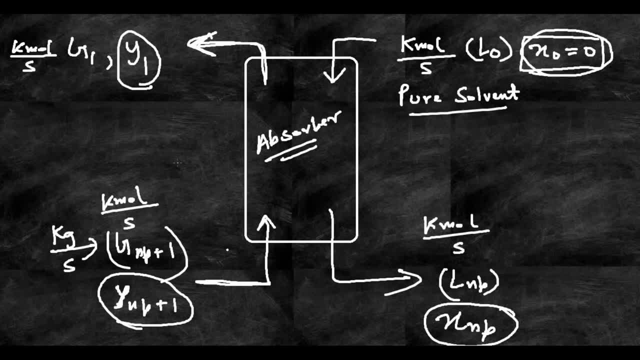 while deriving the equation. also, one more thing that we need to know is so in this equation, or in this diagram, you can see that this capital, g and p plus 1, this g, 1 and this l naught and this l and p, all these are total flow rates, that is, the total kg per second. 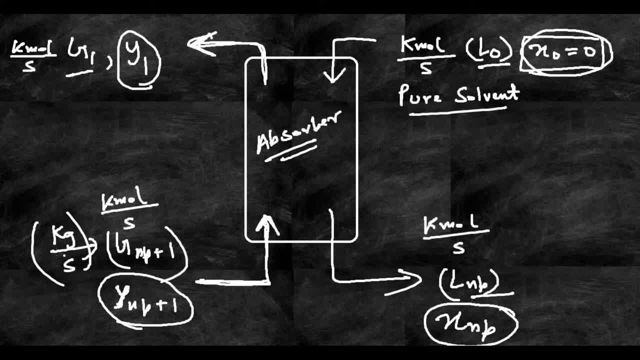 which is entering from the bottom. it does not discriminate whether it is ammonia or air separately. it is the entire thing which is going in. so now my solute is the mixture which i am sending is ammonia and air, and now i will explain you how to do this. so let me tell you exactly how. 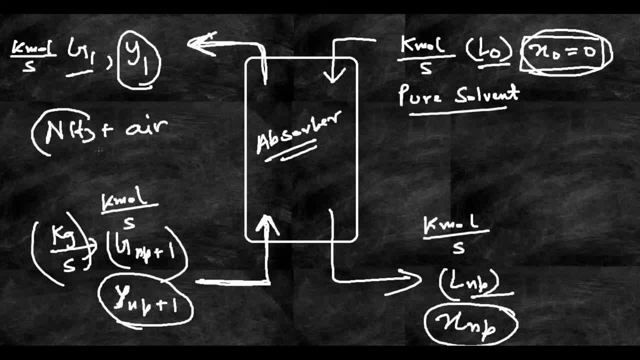 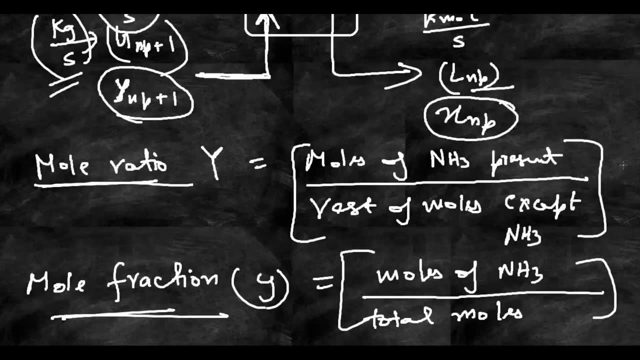 ammonia: ammonia plus air, so ammonia is the solute. i need to absorb this using the water. so now this is the solute. so if i want to calculate, if i want to calculate this flow rate, that is, this kgs per second or kilomoles per second excluding this ammonia, then i need to do a mathematical. 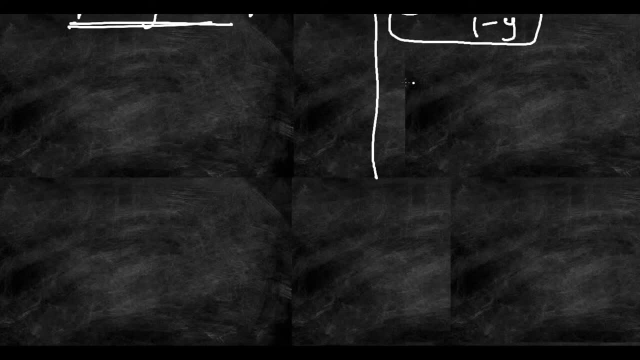 modification. what we will do is: i know that the total rate, the total rate is gnp plus one. this is the total rate, so now, in order to convert it into solute free basis, i need to represent this as gs. so what is so? what is the relationship between this solute free feed rate and this? 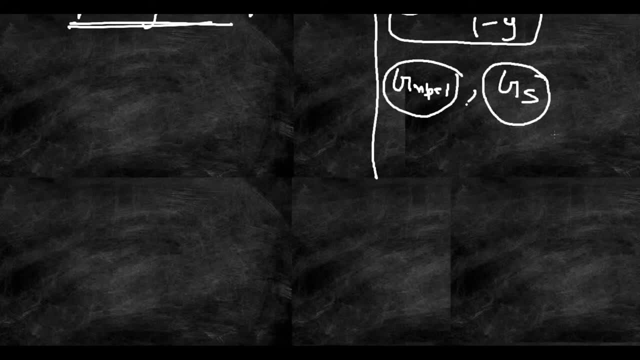 total feed rate. so, in order to find the relationship, the relationship is very easy. it is gs. gs is equal to gnp plus one, where gnp plus one is the total feed rate, times times one minus one, minus y np plus one. so if i do this, if i do this, what i will get is the flow rate, the flow rate, and i exclude the 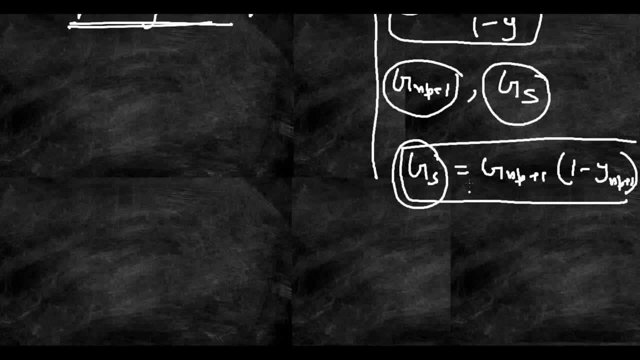 ammonia from this part. why i am doing this? this will be useful while finding the operating line equation. that is, this gs is the kgs per second- kgs per second of air entering where no ammonia is present. this gs is the kgs per second of air entering from the bottom. air entering from the. 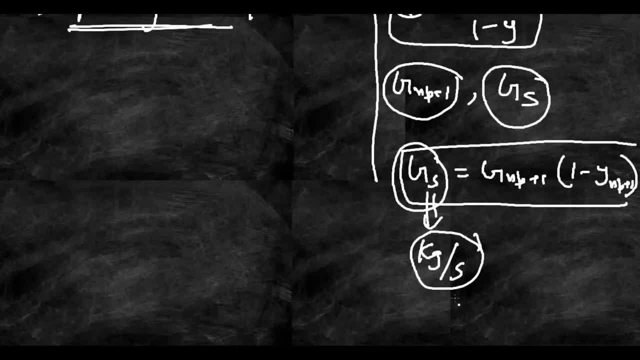 bottom, air entering from the bottom, and no ammonia is present here. no ammonia is present in this gs calculation, while the gnp plus one contains both ammonia and air. this gnp plus one is also in kgs per second, or it may be in kilomoles per second, doesn't matter. 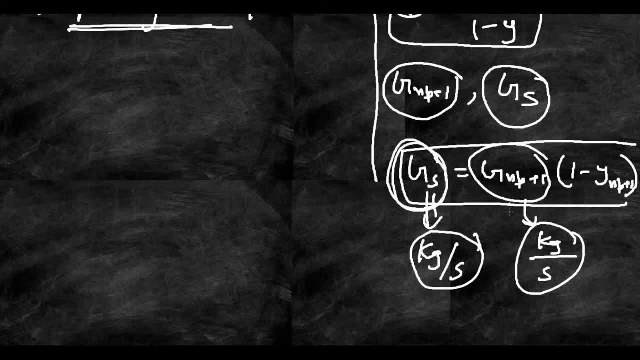 what matters is this gnp plus one takes into account of both air and ammonia, but this gs takes into account only air. it excludes the solute. so this is what is important. so now another thing is: this gs is constant throughout. this gs will be constant throughout, because air is not. 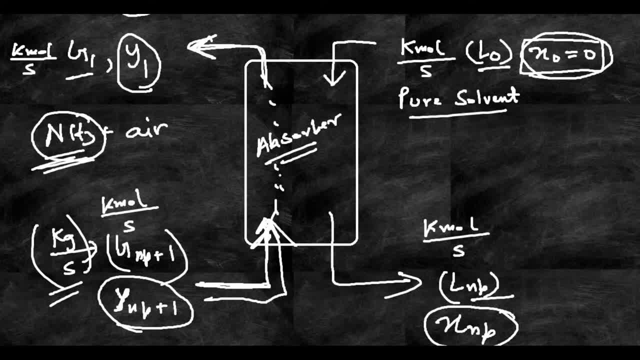 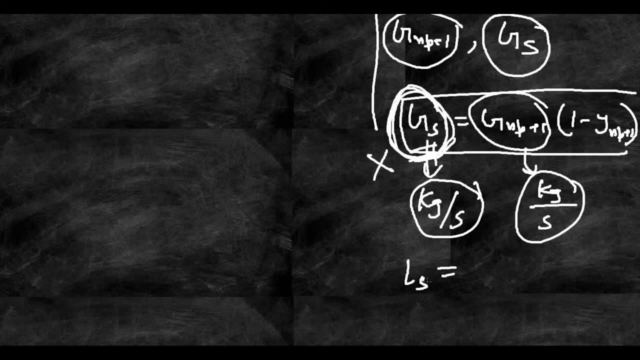 getting absorbed. what is getting absorbed is ammonia, so air flow rate, that is, the kgs per second of air, will be constant throughout the tower. so i can do the same thing for this solvent. i will write this as this: l naught will be written as ls, so ls will be the solute free water, so solute free. 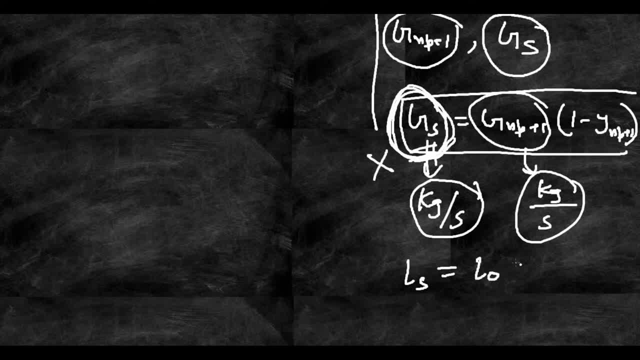 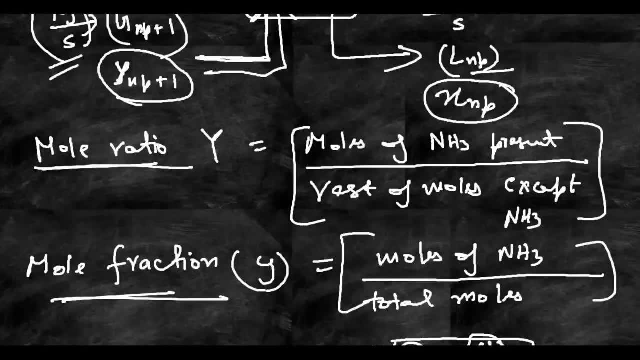 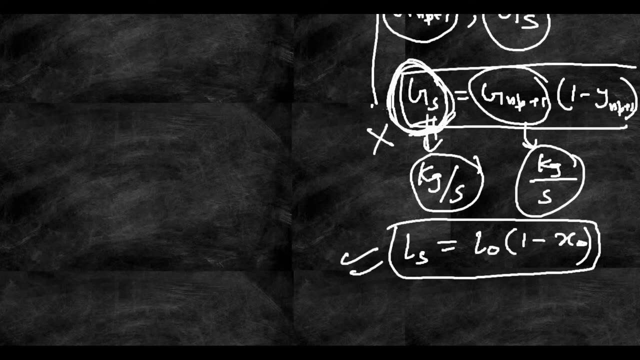 water ls will be equal to the l naught, which is entering times one minus one, minus the mole fraction, that is, x naught. we know x naught is zero, but for the sake of math we will consider it one minus x naught. so this is what we have over here. so these two equations will be useful, these two. 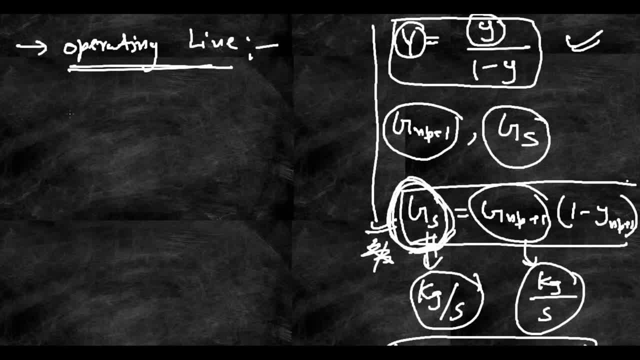 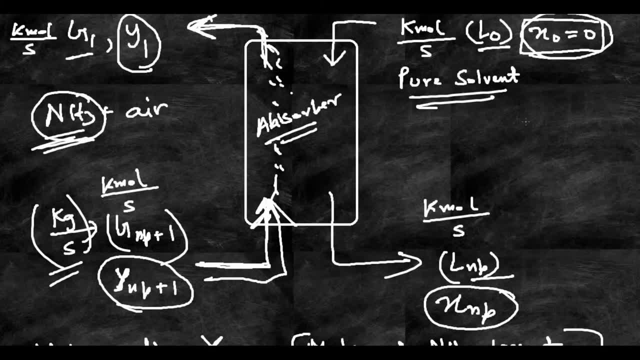 equations will be very useful while deriving the operating line equation. so now to derive the operating line equation, what we will do is we will consider this entire thing and we will take a material balance. so if i take material balance, the things which are entering the absorber, i will 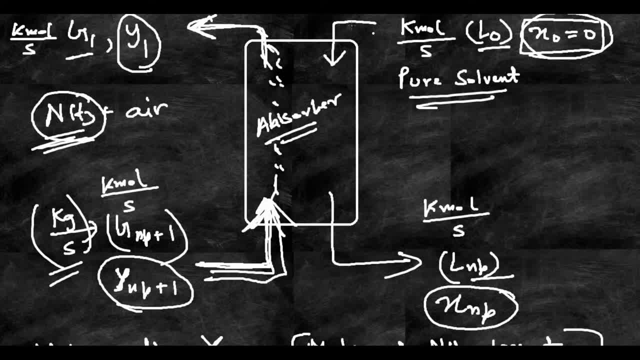 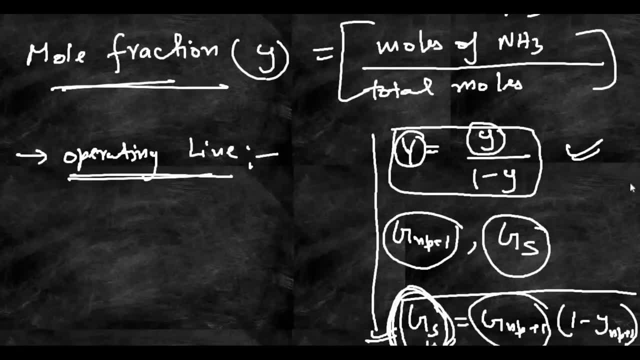 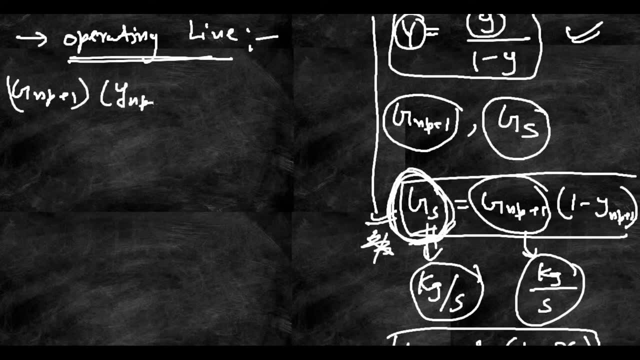 write first. so first this gas stream is entering and this liquid stream is entering, so ammonia in into ynp plus one. so let me write it down: gnp plus one, gnp plus one into ynp plus one, ynp plus one. this ynp plus one is the mole fraction, remember it. so this one is entering, plus also what is entering? 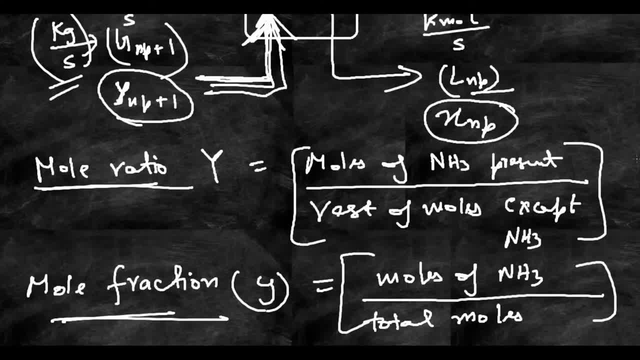 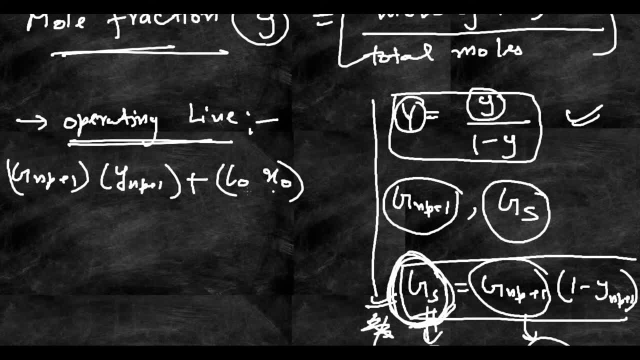 is this, uh, solvent. so l naught times x naught. l naught, l naught times x naught. this is also entering. so i know that x naught is 0, but for the sake of math we will consider it because sometimes little ammonia which is present in the solvent. so to consider it, we are taking this term: l naught. 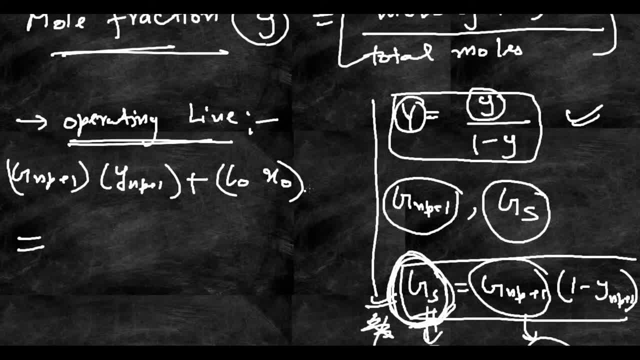 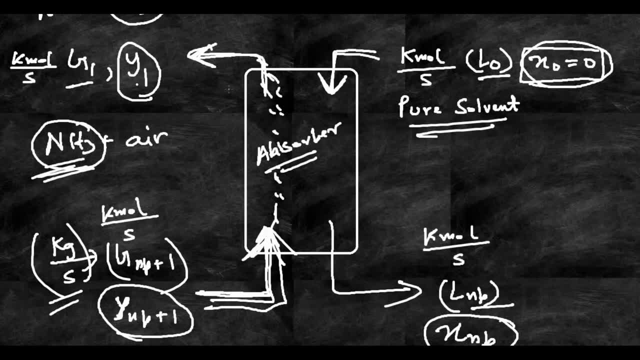 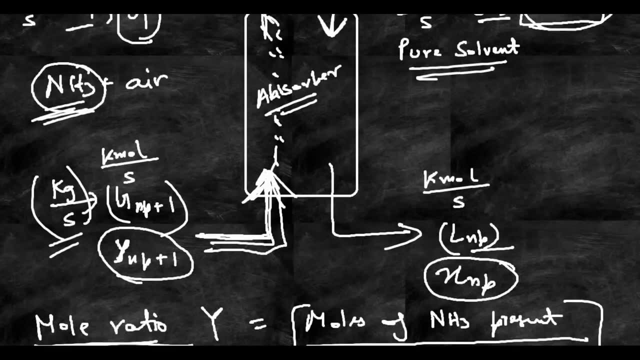 times x- naught. so this is equal to this. x naught is also the mole fraction of ammonia in the liquid stream, so this will be equal to the output. so what is going out? what is going out is g1- y1, so g1 times y1 is equal to g1 times y1 plus g1 times y1, plus lnp times xnp, lnp, lnp, lnp times xnp. 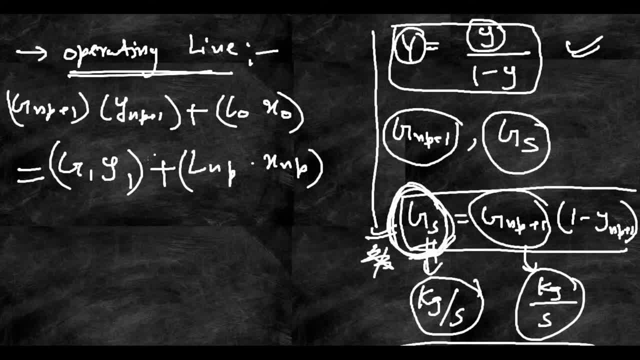 so this is the important equation that we need. this is the equation from which we will derive the operating line equation. so now, what we know is: so now we will con convert this gnp plus 1 into the solute free basis. so if i do this, what i will get is gs. so if i write gnp plus 1 in terms of gs, 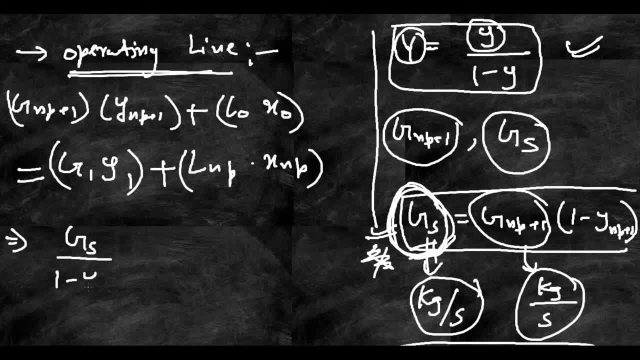 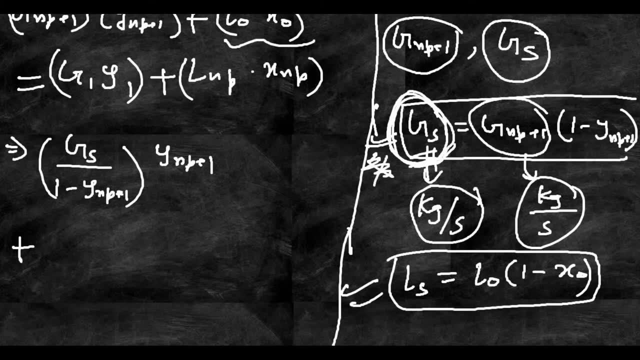 it will be gs divided by 1 minus ynp plus 1. now i multiply this with ynp plus 1, so i will draw a line to separate these two boards. so ynp plus 1 plus plus. i have to take this l naught x naught, so again. 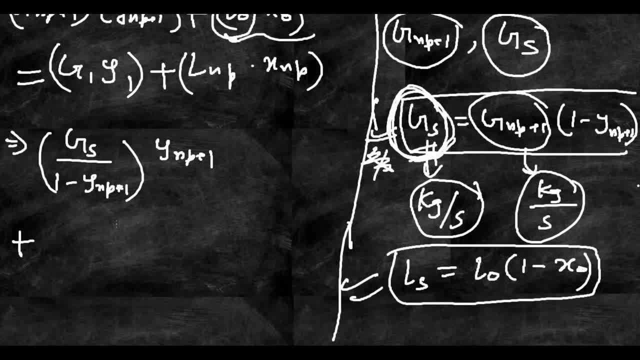 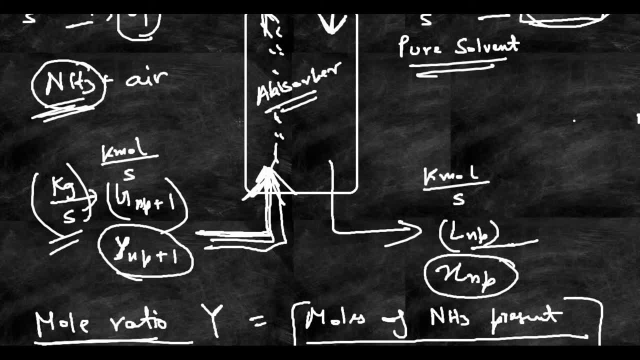 i will represent this. l naught with solute free basis. why i am doing the solute free basis? because the solute free part will be constant throughout the tower. the, the terms considering the entire thing will vary, but the solute free terms, the concentrations, will not change, so i am taking the 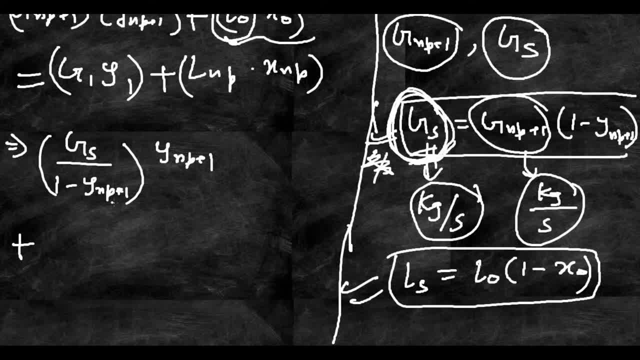 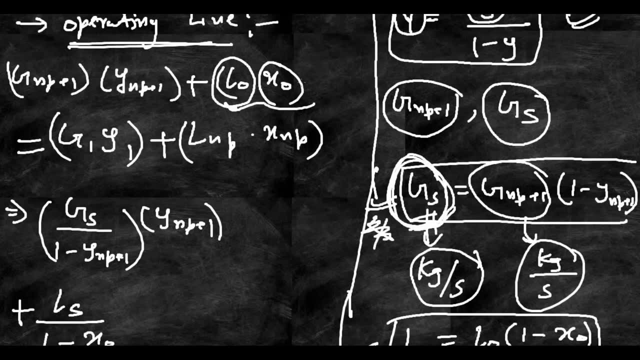 balances without the solutes. so gs by 1 minus ynp plus 1 times ynp plus 1 plus l naught, x naught. so what i will do with l naught, x naught. this l naught can be written as ls. ls by 1 minus x naught times. i have an x naught over here which i have to multiply. 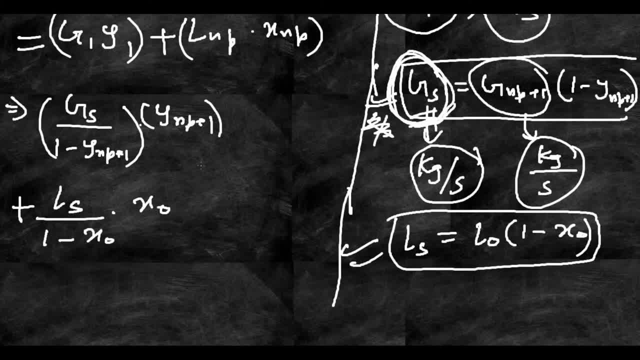 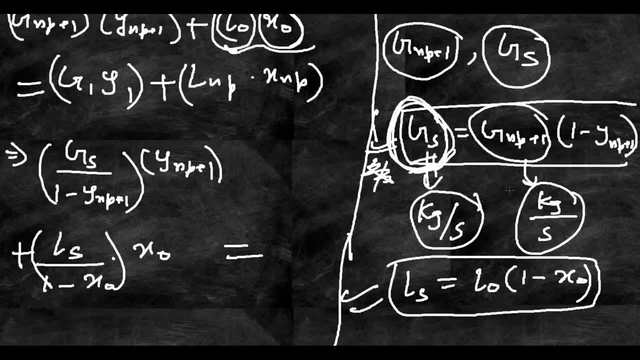 so i multiply this x naught. so this is on the left hand side of the equation. this entire thing is equal to. this entire thing will be equal to. what i have to write over here is g1, y1, so g1 will be written as g1 will be written as gs, gs. 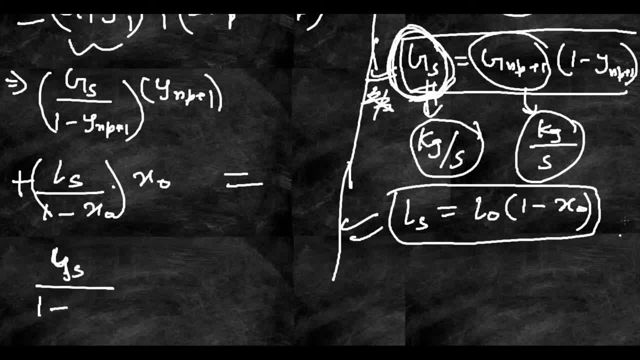 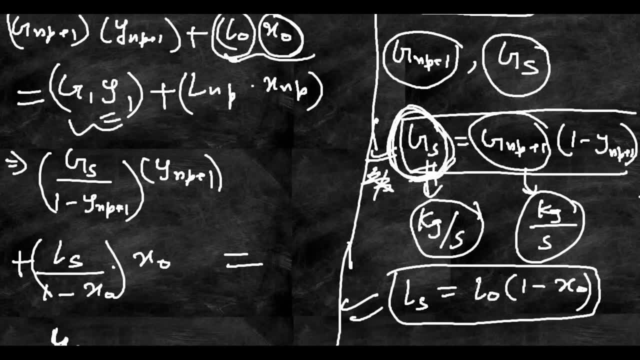 divided by 1 minus gs, divided by 1 minus y1, 1 minus y1, and there will be a y1 which i have to multiply this y1, so it will be gs by 1 minus y1 times y1. so this is what i have. 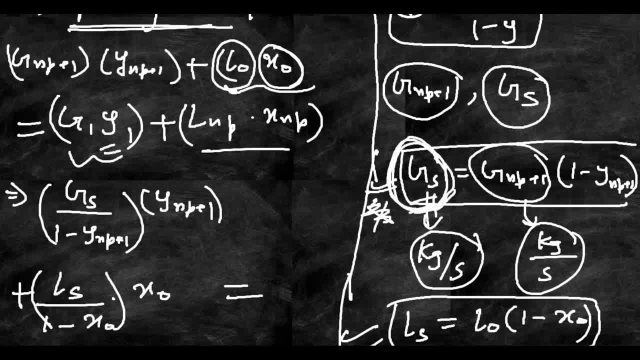 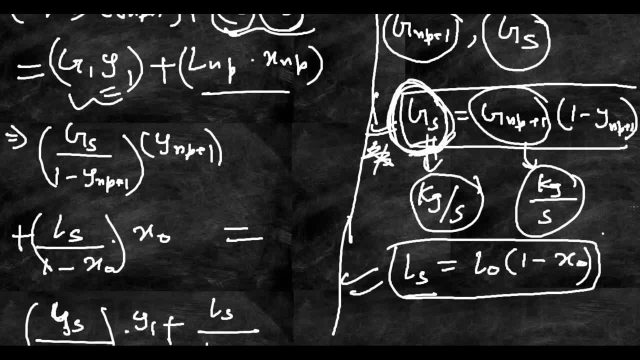 plus plus. i have another term, which is lnp times x np. so this lnp can be written as: ls divided by 1 minus ls divided by ls divided by 1 minus x np. 1 minus x np. Why I am having xnp over here. 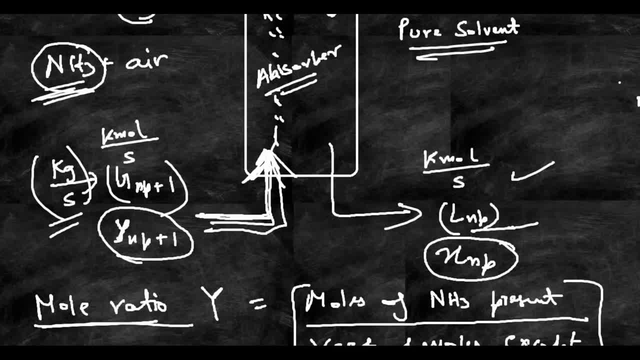 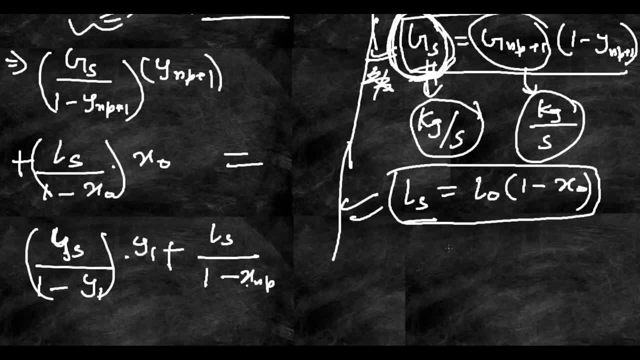 Because I am talking about this stream. I am talking about this stream. When I am talking about this stream, I will take x0.. When I am talking about this stream, I will take xnp. So ls by 1 minus xnp and I have to multiply this xnp also. 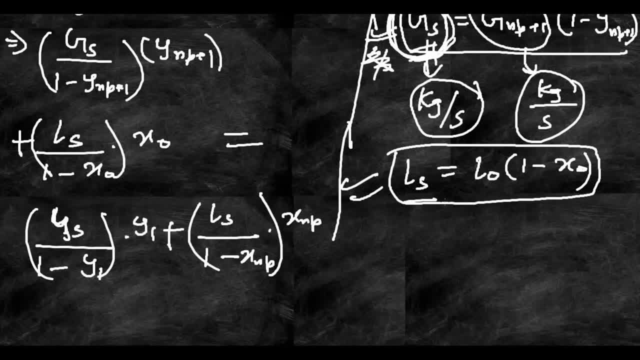 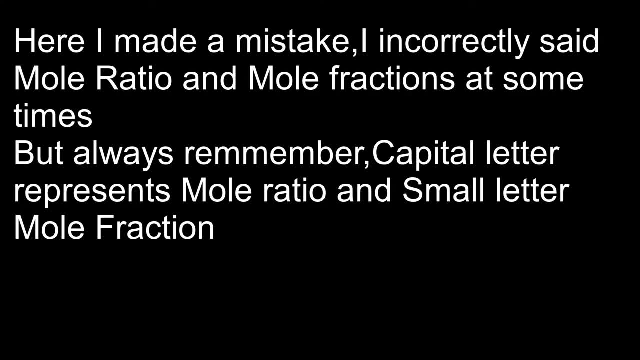 So multiply the xnp. So this is what I get. Now you can see over here I have a relationship between mole ratio and mole fraction. Mole ratio equals to mole ratio divided by 1 minus mole ratio. So you can see over here I have mole ratio divided by 1 minus mole ratio. 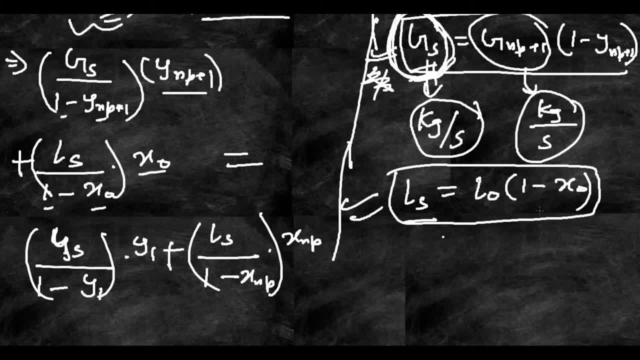 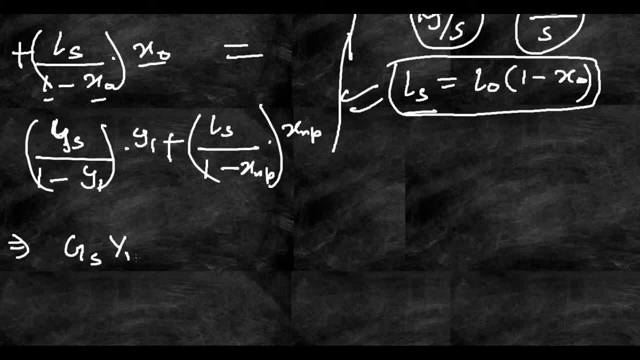 Again mole ratio divided by 1 minus mole ratio. So I will convert this into mole fractions And what I can write is this: can be written as gs, gs times ynp, But ynp plus 1.. Notice that I have changed from small letter to capital letter. 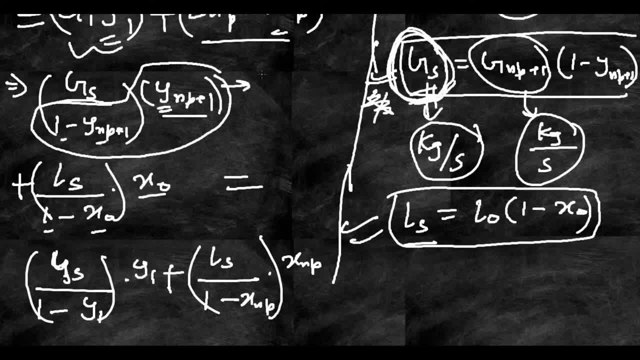 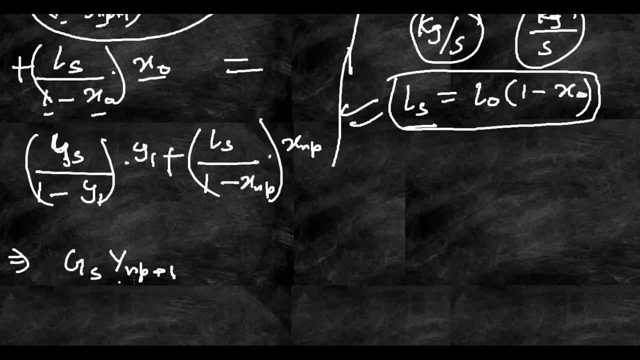 Because I have taken this entire term. This entire term is my capital ynp plus 1.. Which is the mole ratio. So I will do the same for all the things And what I will get is gs times ynp plus 1 plus ls times capital x0.. 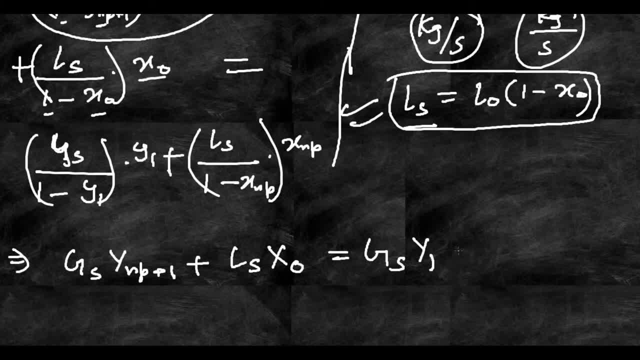 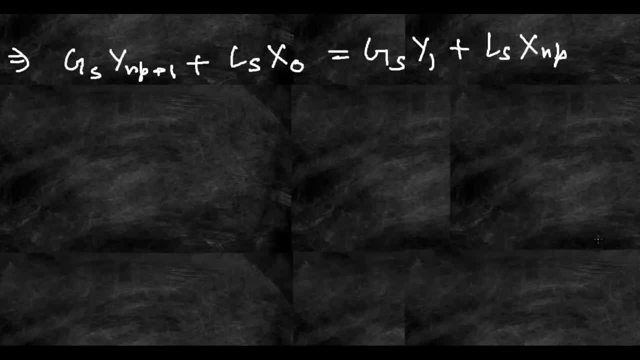 Is equal to, again, gs times capital y1 plus ls times capital xnp. This is what I get, So now I will simplify this equation. I will take the gs terms on one side. So gs terms gs times ynp plus 1 minus y1 equals. 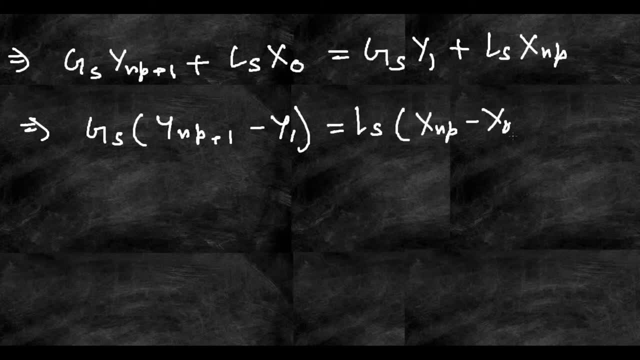 ls lx times xnp minus x0.. This is what I have. So, from here, what I can write is: ls by gs, ls by gs equals to ls by gs equals to ynp plus 1 minus y1.. 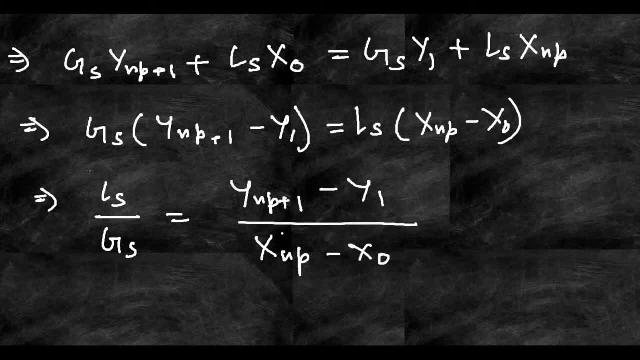 Divided by xnp minus x0.. So this equation is very important in solving most of the absorption problems, Because this is the equation of the operating line, This is the equation of the operating line, Equation of the Operating Operating line. 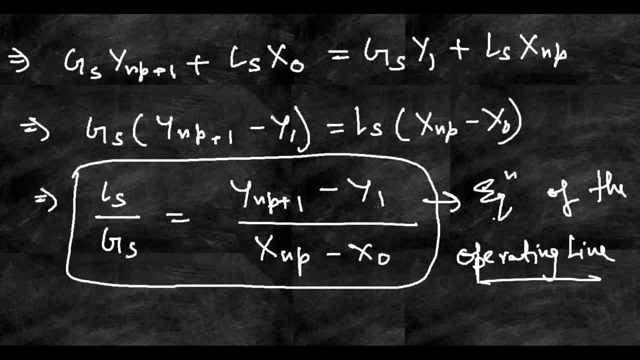 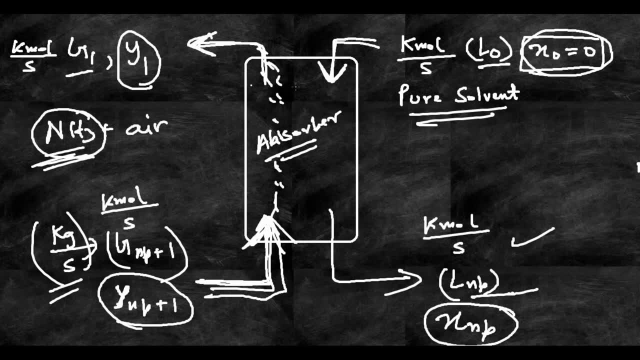 Equation of the operating line. So now we will see how to plot this and determine the number of stages which are required to do this absorption. We will be calculating, We will be calculating the number of trays which are required within this absorption tower in order to do the required absorption. 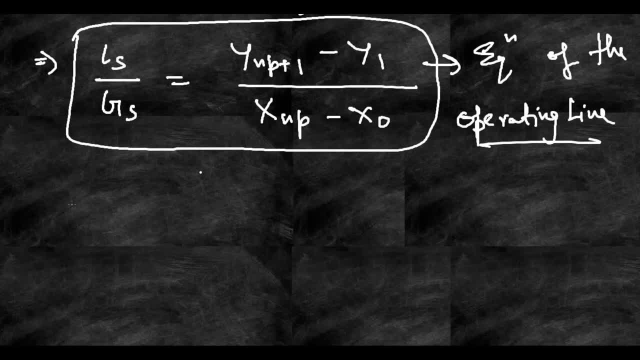 So, to do that, what we need to do is we need another line, which is known as the equilibrium line. This is the equation of operating line. Another line which we will need is the Equilibrium line. Equilibrium, Equilibrium line. 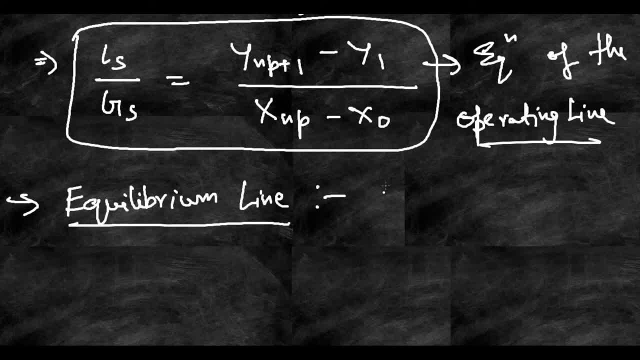 So this equilibrium line data. it will be provided to us. In most of the cases, this equilibrium line data is provided to us. It is given to the basis of ammonia water, Ammonia water solubility. In this ammonia water solubility, an equilibrium data will be given to you. 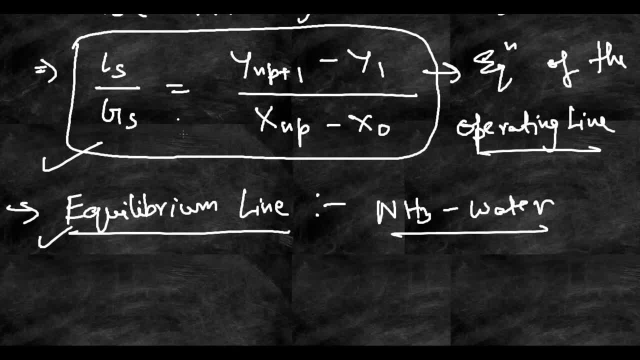 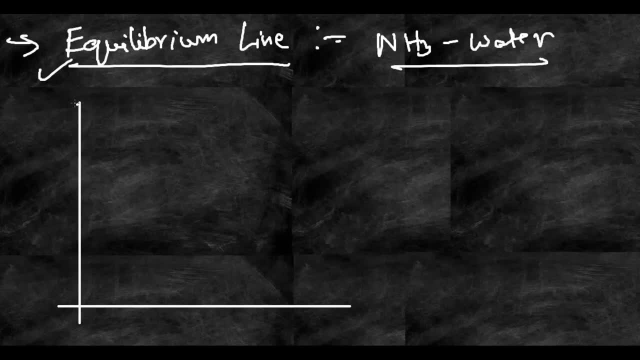 So now what we need to do is using these two. we can plot and calculate the number of stages. I will show it to you. Ammonia- water solubility. So in this graph, I will plot the mole ratio of ammonia in the gas stream. that is the. 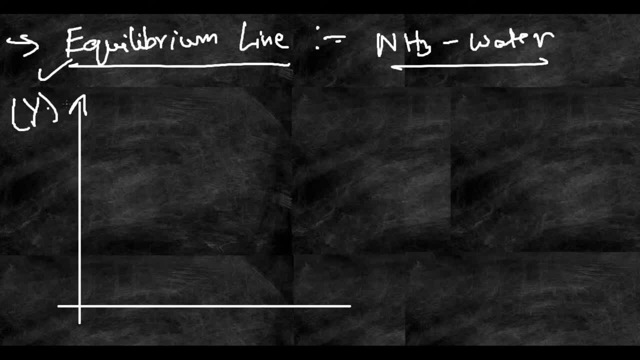 capital Y, The mole ratio of ammonia in the gas stream. that is, capital Y will be plotted on the Y axis. And capital X, that is the mole ratio of ammonia in the water that is in the liquid phase, I will plot it on the X axis. 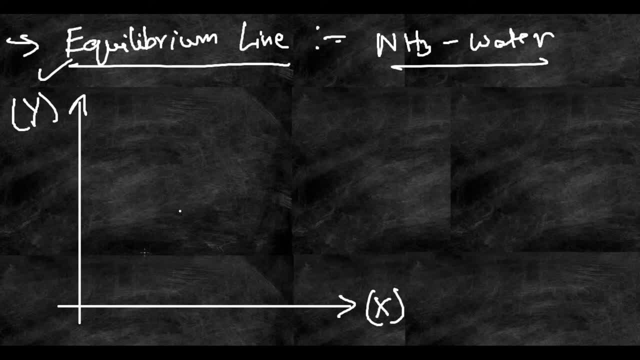 So this is the graph that I have. So first, the equilibrium line will be given to us. So if the equilibrium line follows a linear relationship, then we will get a straight line like this: we will get a straight line like this if the equilibrium line follows: 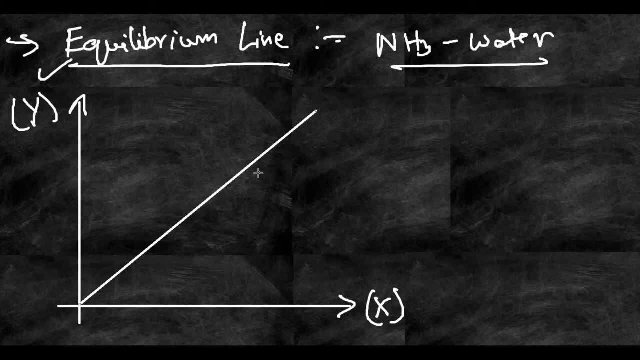 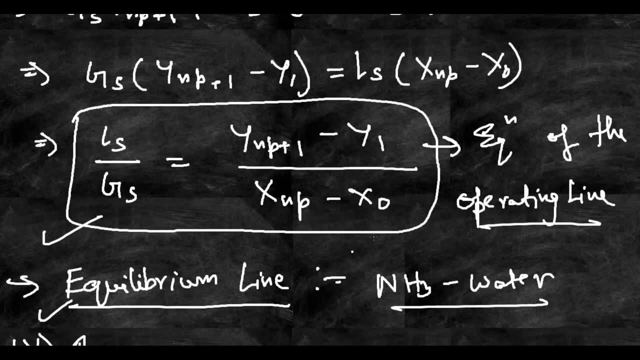 a linear relationship. So, to make this simple, we will consider that the equilibrium line is a linear relationship. Now we will try to draw the operating line. You can see that this operating line is also a linear line, that is, a straight line equation. 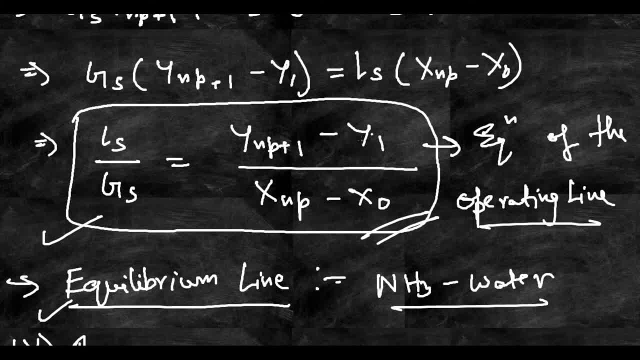 So first, what we will do is we will calculate this Y1.. The first point is Y1, Y1, X0. First point is Y1, X0. So how to do this, We know. I have said before. 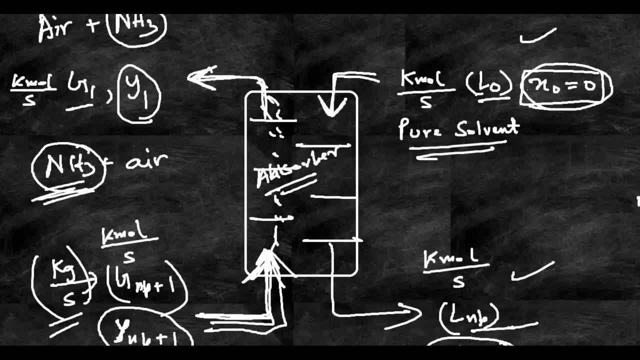 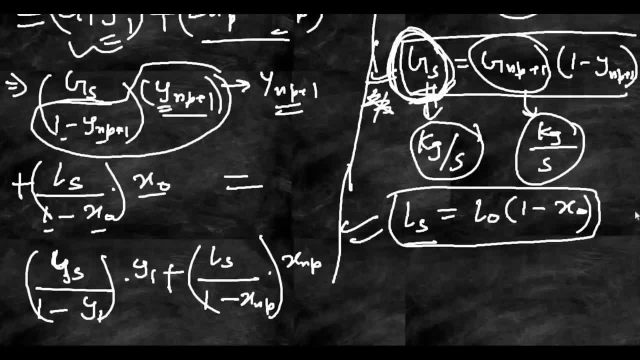 So how to do this? We know that the water which is entering from top the X0 is 0, because this water will not contain any ammonia. It is a pure solvent. So for pure solvent, what will happen? This X0 will be 0, this X0 will be 0, but there will be some value of Y1. 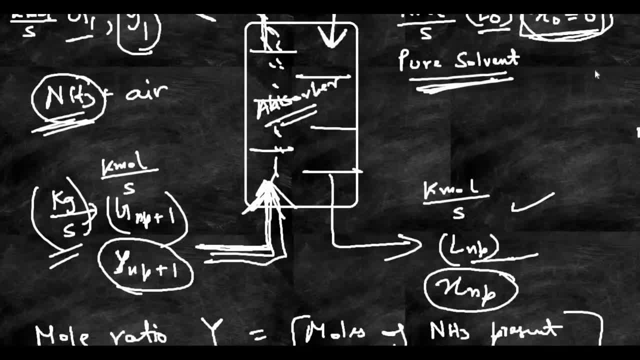 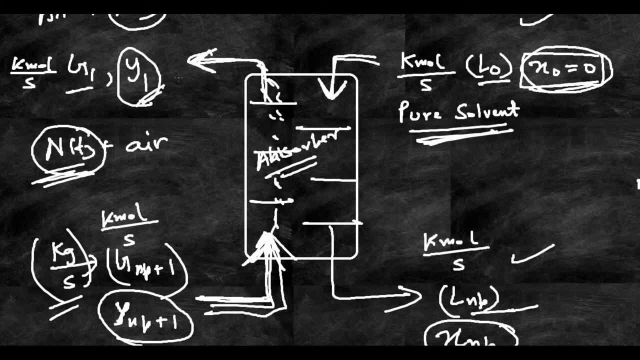 There will be some value of Y1, because Y1 is the ammonia. Y1 is the ammonia which is leaving from this gas stream. We know that absorption has already taken place, but still some amount of ammonia will be remaining in the outlet gas stream. 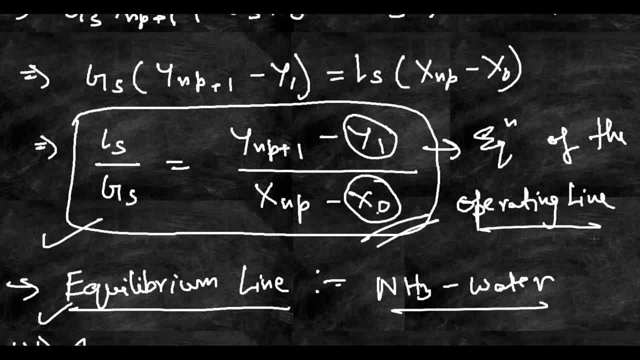 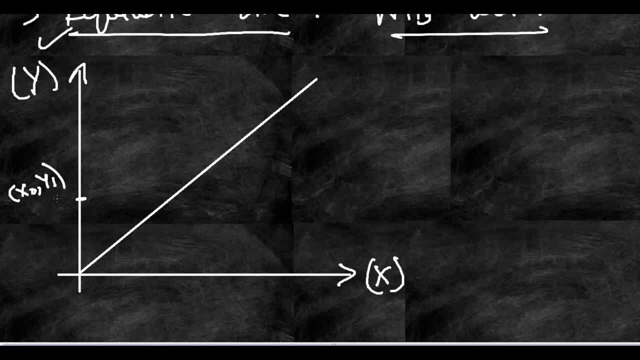 So that will be that Y1.. So I have the first point, which is X0, Y1.. So I will plot it over here. So let this be over here: X0, X0, Y1.. This is my first point. 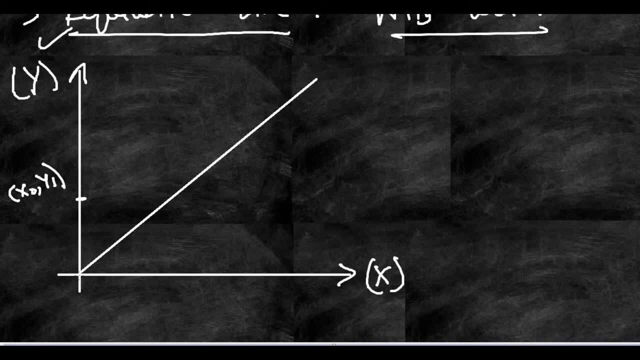 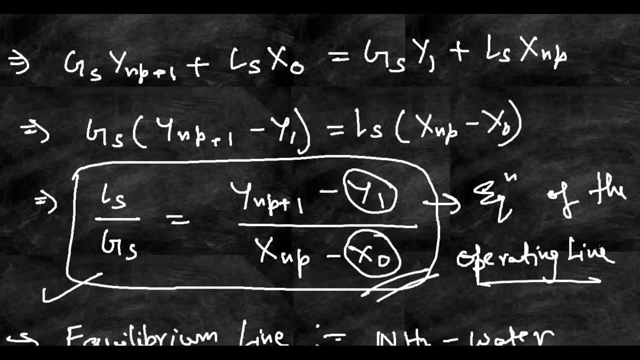 So X0 is 0. I have assumed X0 to be 0. That is why the point is located on the Y axis, because X0 is assumed to be 0 over here. Now, the second point through which this operating line will pass is the Ynp plus 1 and Exnp. 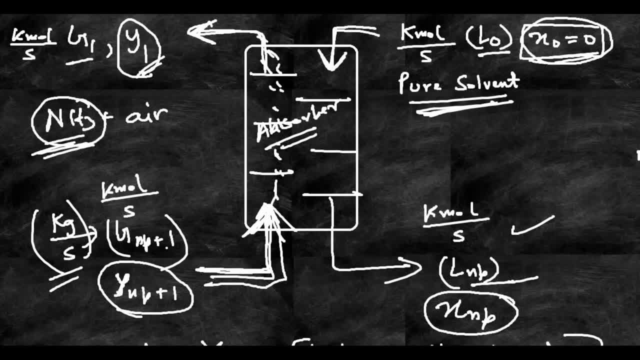 Notice that Ynp plus 1 is the mole ratio of ammonia which is present in the X0.. So what we do is we will plot this there And then we will write it. So let me write down my first point here.